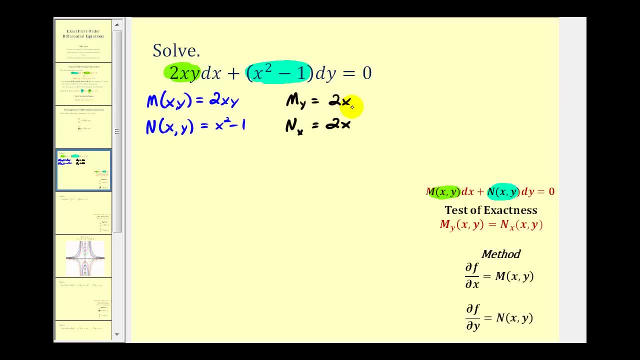 minus 1 with respects to x would also be 2x. So this means we do have an exact differential equation, which means our solution will be: our function f of x comma y equals a constant c, and we can find our function f of x comma y using these two. 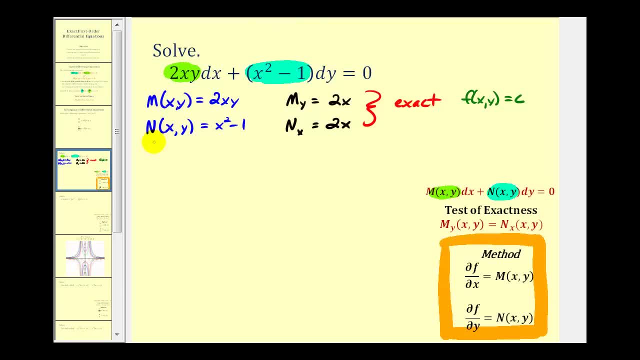 equations here. So if we know the partial derivative of f with respects to x must equal m of x comma y, then if we integrate both sides of this equation with respects to x, we'll recover the x part of our function. f of x comma y, which means f of x comma y, must be equal to the integral of m of x comma y, which is 2xy with. 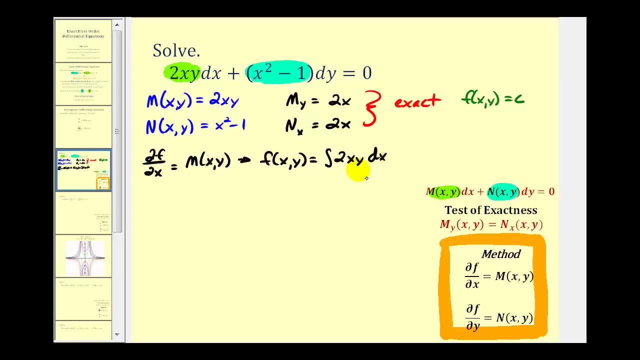 respects to x. Now keep in mind when we integrate here, because our function f is a function of two variables, we'll only be recovering the x part of this function. So f of x, comma y is going to be equal to integrating with respects to x. we would have 2 times x squared divided by 2.. So the 2's would simplify out. so we'd have x. 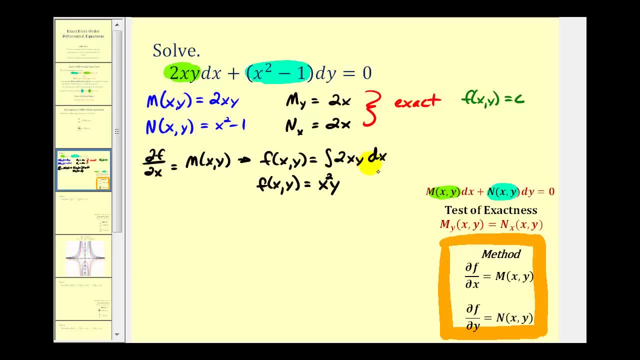 squared y, But then to show we've only recovered the x part of the function, not the y part. we'd have plus a function of y. let's call it h of y. So now, if we can find h of y, we'll have f of x comma y, and therefore we can find our solution to the. 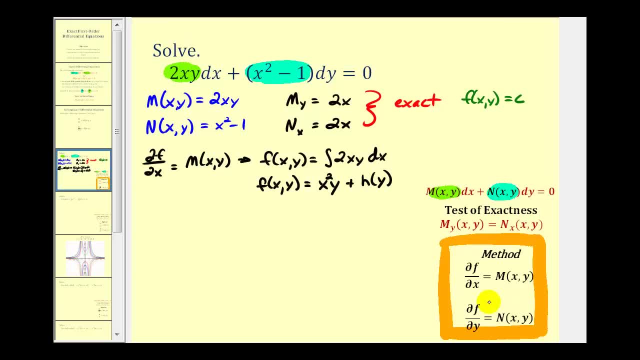 differential equation. So now we use the second equation here, where we know the partial derivative of f with respects to y must equal n of x comma y. So what we'll do now is we'll find the derivative of f with respects to y and set it equal to n of x comma y, which we know is x squared minus 1.. So here's our 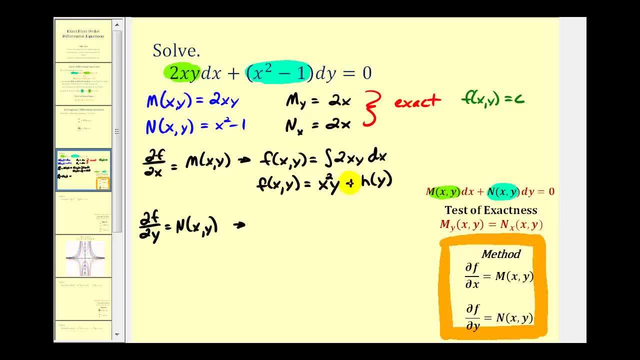 function f, and now we'll find the derivative with respects to y. so we'll treat x as a constant. So here we would have x squared plus the derivative of h of y, which would just be h prime of y, And again this must equal n, which is x squared minus 1..